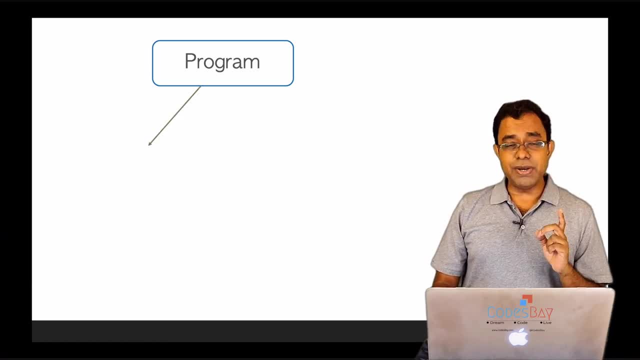 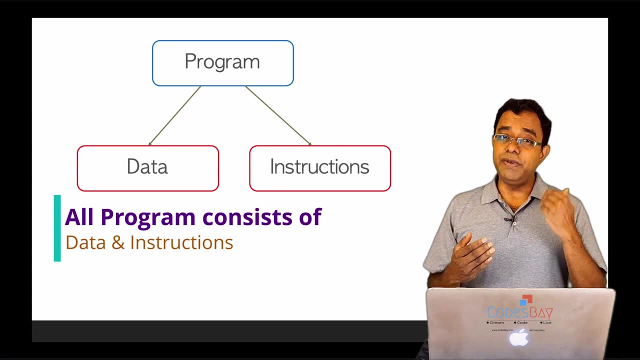 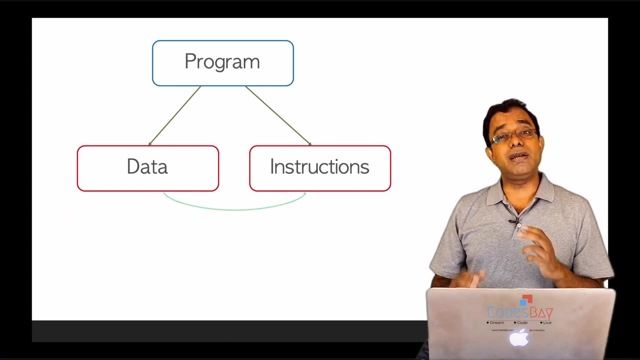 Any program consists of two things. Thing number one is data, Thing number two is instructions. All the programs we have written or we will write consist of two things: data and instructions. The instructions require data to do something. For example, if you want to sum two numbers, you need to provide data, two numbers, so that these two numbers can be summed. 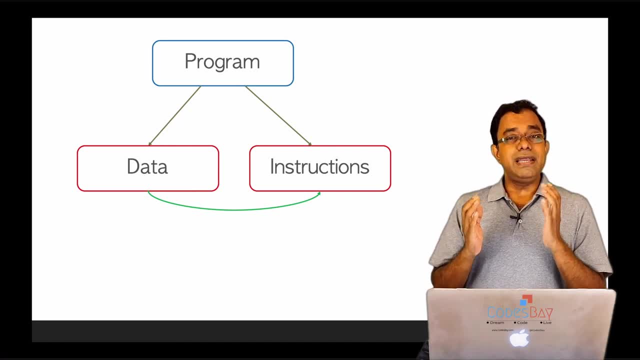 Clear Right. So, similarly, we need data for instructions. So not all data set is required for execution of instructions, For example, sorting, searching, storing in database, retrieving from the databaseor- for that matter, storing the state machine information. What happens is there are a set of instruction sets which either retrieves or stores large amount of data. 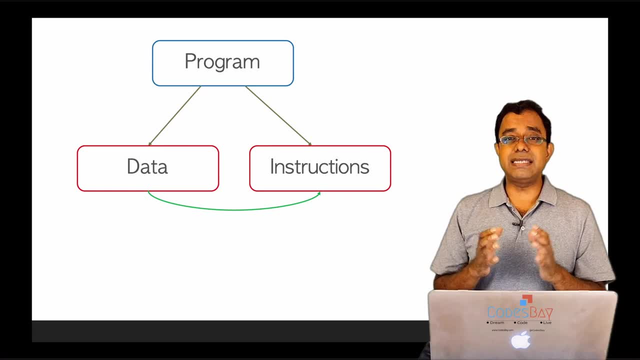 So now we know that instructions require that data, So so that researchers are going to be able to come up with some very nice ones. instructions access data which is generally stored in memory. If it is not stored in memory, then what will happen? It will take lots of time, And that is the main reason why in-memory. 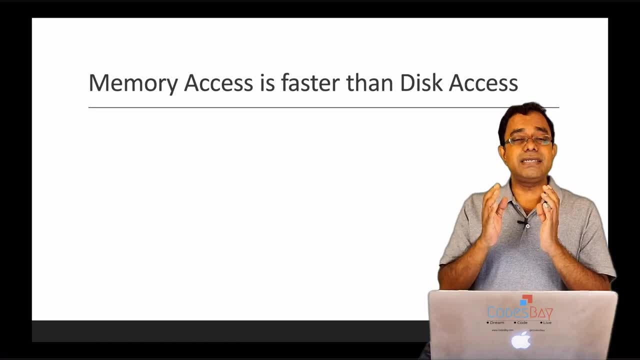 databases are very, very helpful because accessing something from memory is much, much, much time faster than accessing something from desk, And we are doing the same for quite a long time. Think about linked list. What was a linked list? It just stores data in. 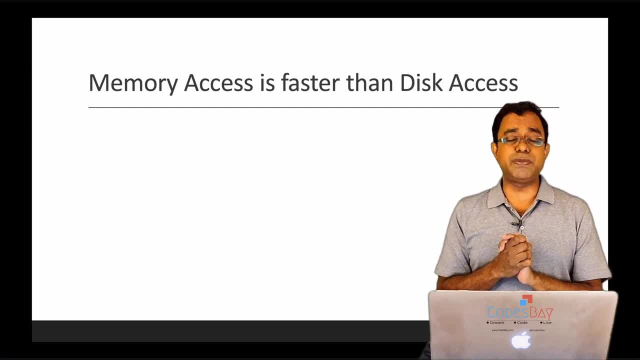 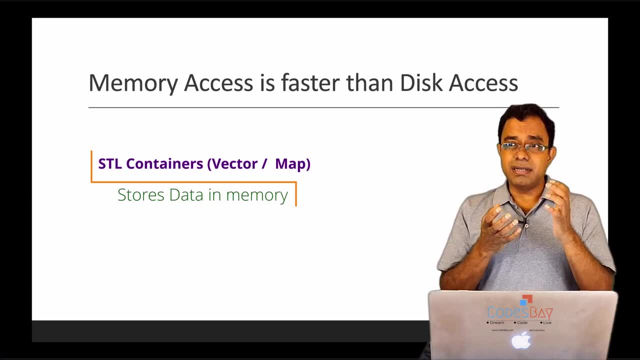 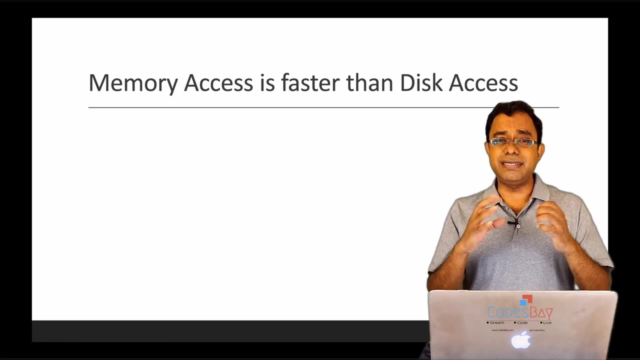 the memory so that we can access. If you are a C++ programmer, think about what are HDL containers, vectors, map DQ. They are just containers for storing data in memory so that we can access it right. So in here what we are doing: that instead of storing memory. 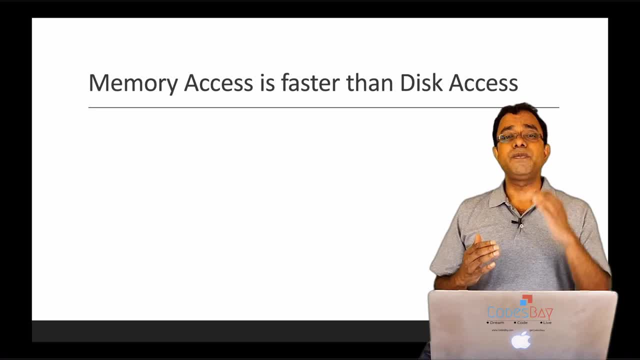 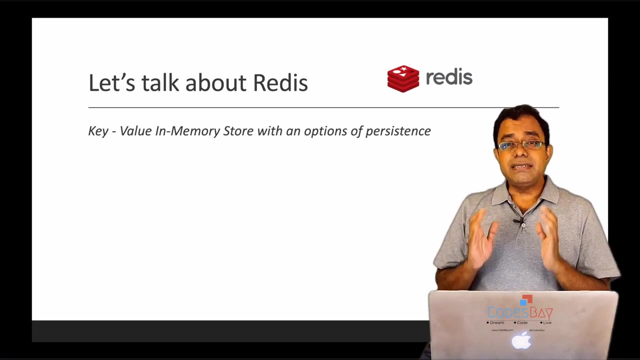 in our own process, in our own data structures, we have something called memory In-memory databases to store the data in in-memory so that we can access it in a faster way. Now let's talk about Redis. What is Redis? Redis is nothing but a key value in-memory. 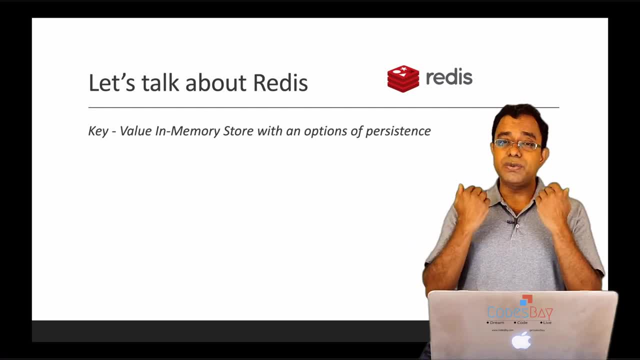 store. It's a key and value. So you store a key and value could be anything. There are various data types about which we will explore in upcoming videos, but just consider it as a key value: in-memory store. Now, it also has a key value in-memory store. So if you have a key value, in-memory store. 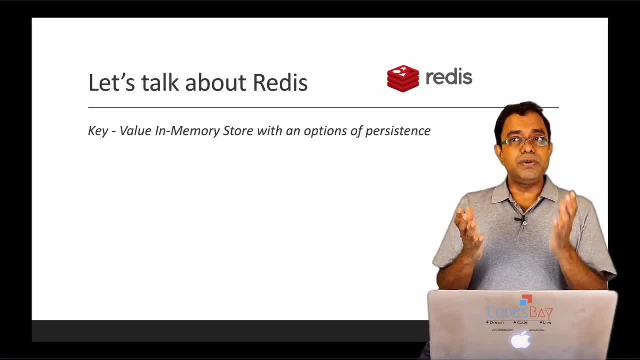 you can use this to store data in-memory, But it also has a option of persistence. So you know that if something goes wrong in the server, or if it is rebooted or for some weird reason, Redis server itself crashes, in that case we will not be able to recover. 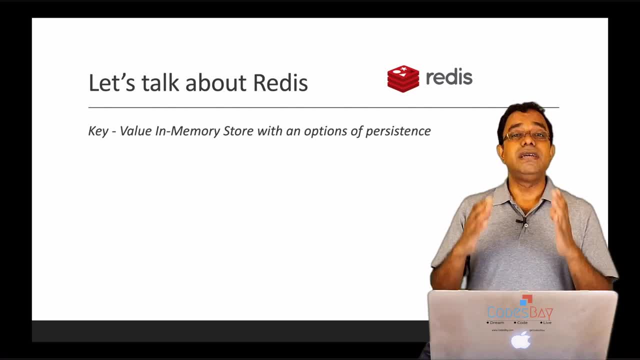 whatever was there in the memory and that may be a loss. That's why Redis also provides a mechanism to store data in the disk for persistence. Now you may think that if you are using a persistence mechanism, the disk will also be able to store data in the disk. 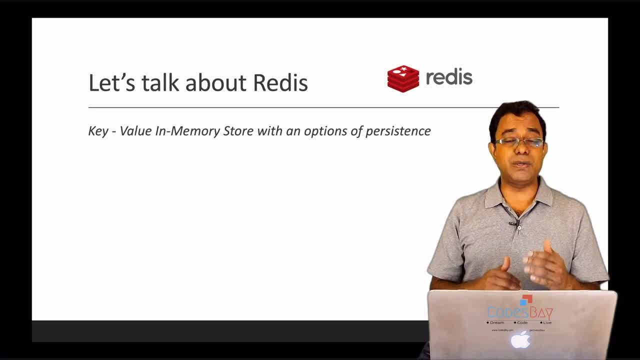 But that's not the case. If you are using this, you will have some problems. The disk database, radius database, will be as slow as any other database. no, that's not a case. there are different ways of doing persistence, for example, snapshot. you can take a snapshot at a different. 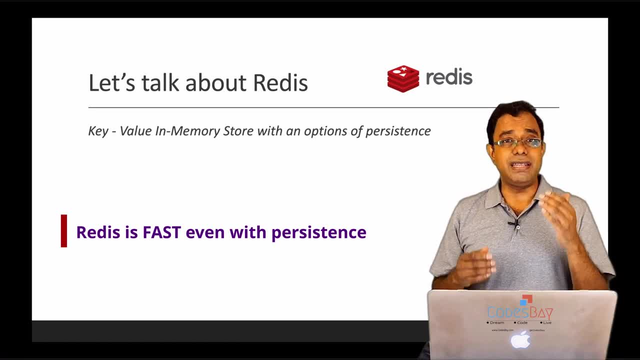 intervals or, for that matter, append only file where anything written onto the in-memory database is also written into the physical database, but at the same time, if you want to read it from in-memory database, it will be fast. okay, now one important thing: redis is primarily a key value. 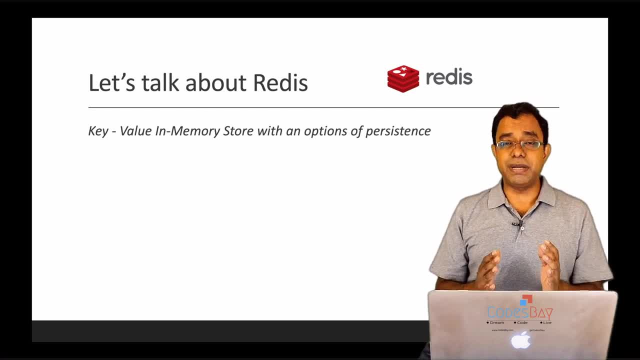 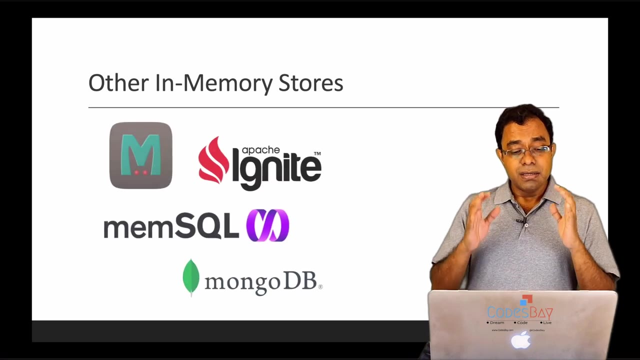 store. but you know what? redis is also a publish subscribe mechanism. redis is also a streaming service. we will talk about all these functionalities of redis in upcoming videos. now let's talk about some of the comparison with other in-memory stores. so some of the things which you are seeing on 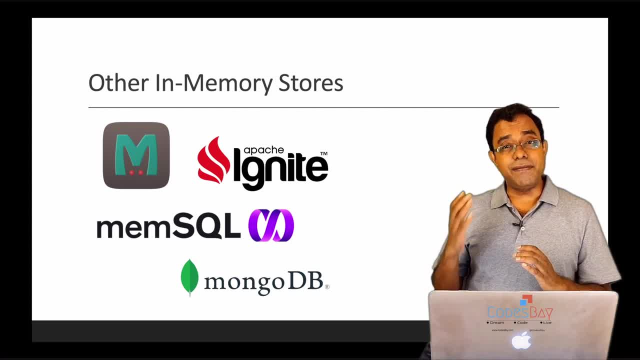 screen right now. they are also in-memory database or are having in-memory variant within them. for example, memcast is a simplest in memory key value store, but data types are limited. apache ignite is also a very nice in-memory data store, but it is much, much more than just a in-memory store. i mean it's a bit heavyweight if 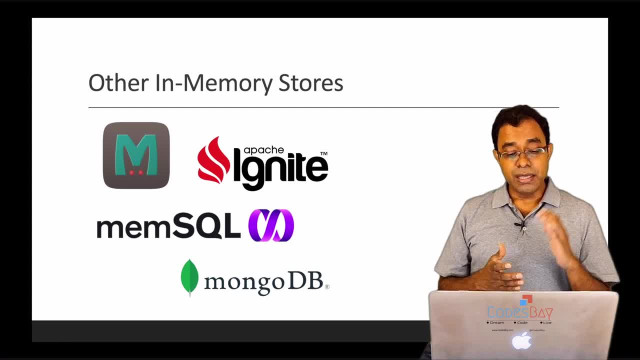 you just want to use a simple in-memory data store. memsql is a sql in memory, so that i mean you can store all the data relationship data in memory, and i think it also provides some free tires, some free uses. mongodb is also having a in-memory engine, but this is unfortunately not available in community edition as of now. it is. 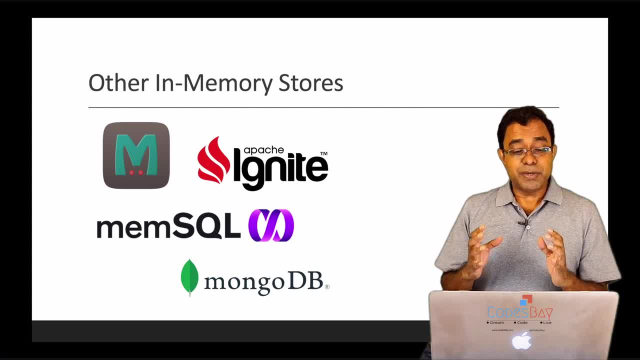 available only in enterprise edition. so these are some of the prominent in-memory databases. there are many other in-memory databases. now, a very important thing: all these databases which you are seeing in your screen are all in-memory databases. so these are some of the prominent in-memory databases which you are seeing in your screen right now. it's good for some specific purpose. 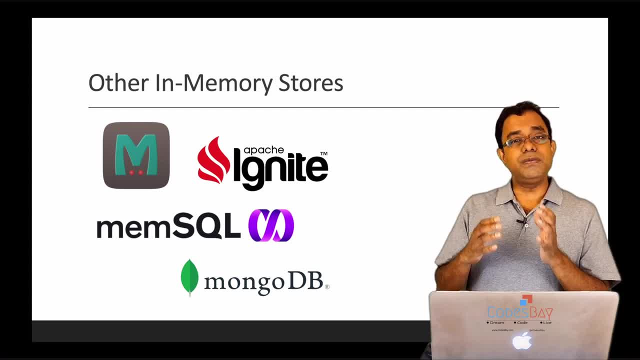 so does redis. okay, as we go through exploring the redis, you will come to know why i talked about redis first, before talking about any other in-memory database. these databases and many other in-memory databases are equally good in many other situations, so there is no one solution fit all. 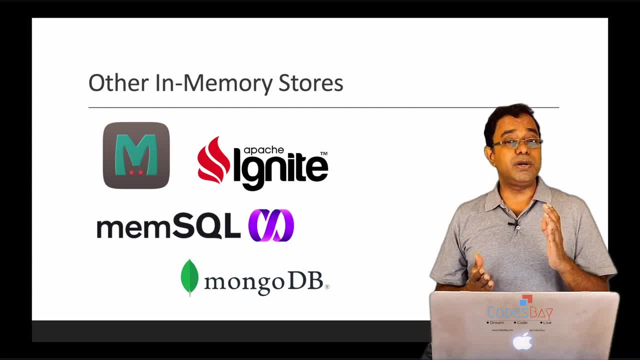 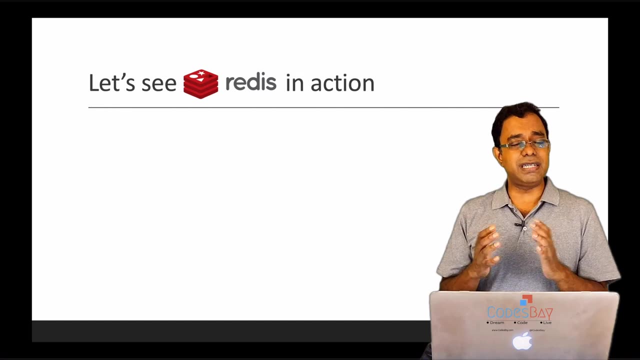 you need to evaluate your database requirement and find out which in-memory database is good for you. most of the situation going forward, okay, so let's see red隨ладئ� in action. i'm not gonna go ahead with download instructions because you know what it's pretty. 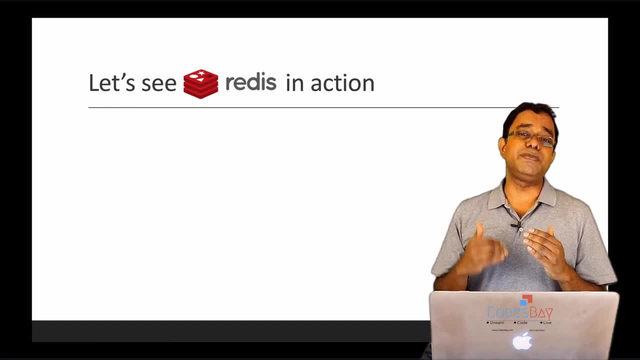 simple. you can just go download and follow four line steps to make it. unfortunately you cannot make it in windows. you can do it in mac and linux, but in windows you can run a docker. so i have already downloaded and installed the latest redis in my mac, so for example, in one device in lingu Galileo. 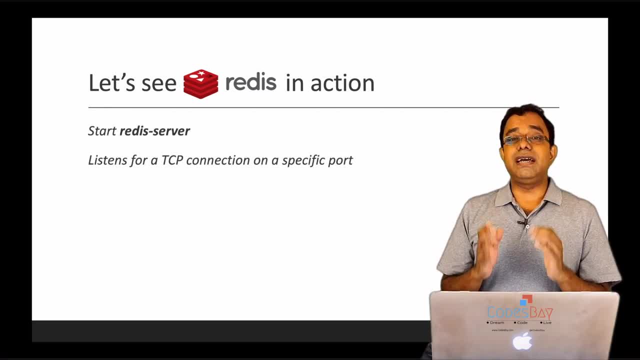 more than Estoyando en줘 recuperando los dlgados para desarrollar los alludedores de Redis de WeEst. no puedo hacer esto en windows. a Evet que en windows, however, you can install the latest dprés America. so to What I will do is that I will use a command given by Redis to start Redis server. 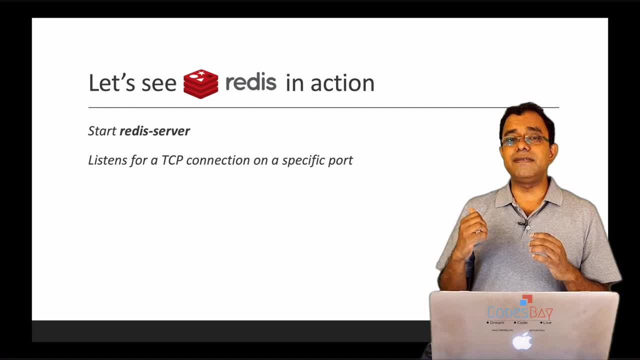 The command is Redis server. It starts a Redis server and listen for an incoming TCP connection on a specific port. We can connect it from anywhere with a local machine or from other machine using the IP port type. The good thing about Redis is that you know the drivers are available in pretty much all prominent programming languages. 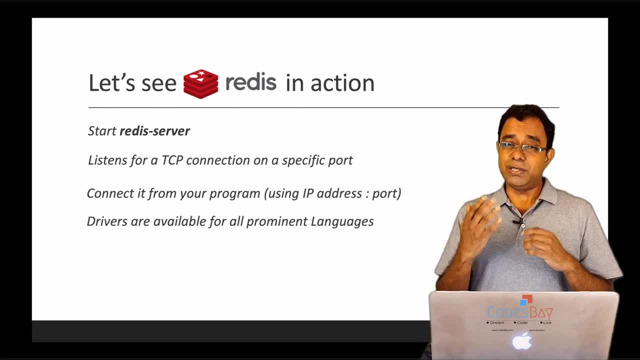 So that you can write program in any language and you have driver to access Redis and send Redis command and get the value, set the values. And apart from all this there is something called Redis command line interface And this is the best way to learn Redis. 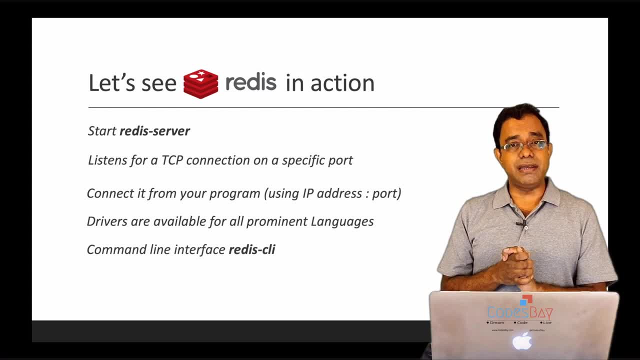 So I will be starting with Redis command line interface. You can use command line interface all the time, whether or not somebody else is also connected to the Redis server. OK, because you know it can accept multiple connections. So let's go ahead and see how we can start Redis and do some basic operations on it. 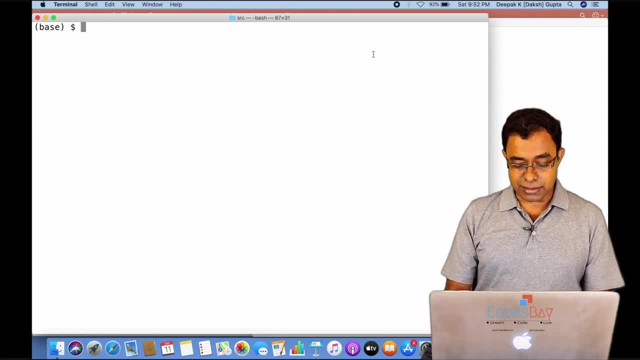 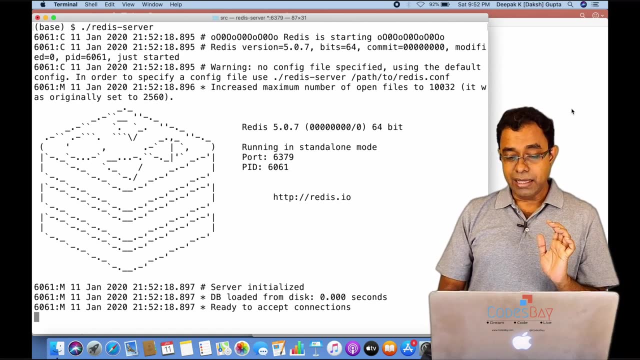 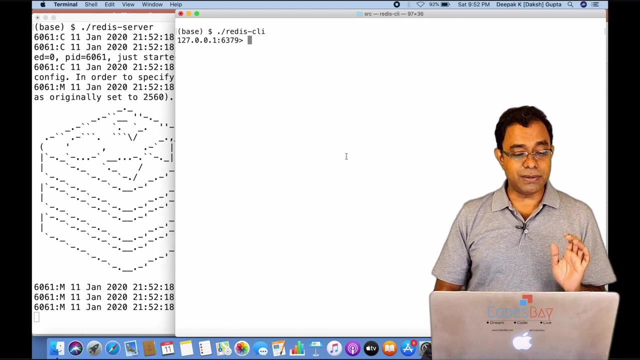 So I am here at my terminal. I will start Redis server by calling Redis server And you can see that Redis server is up and running. OK, now I can use Redis command line interface by calling Redis CLI. Now I am connected to this Redis server. 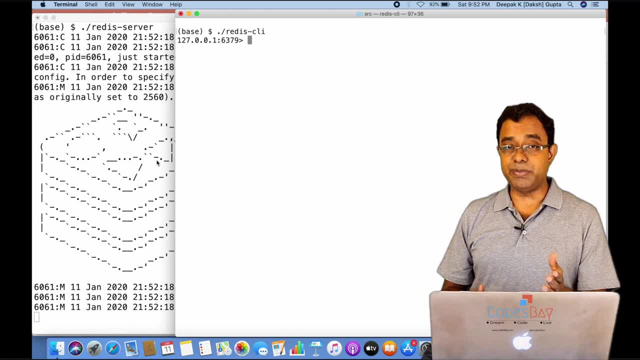 OK, if you are using some driver, you will connect to the same port in the same way. Now, as we know that Redis is primarily a key value store, so we can create a key and a value. So we can create a key like, let's say, first and value is hello world. 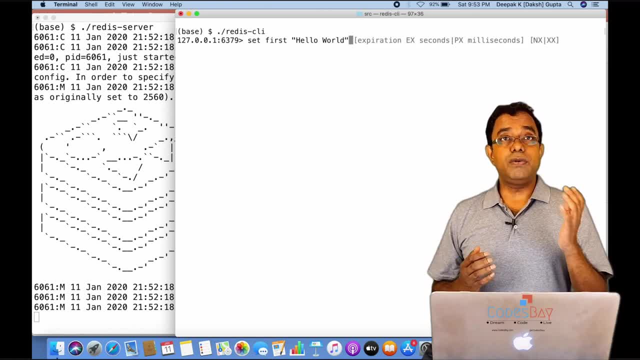 There are various options which we can use about, which I will talk about when I will explain the Redis command. But just for this moment, consider that key value store is set like this: Set key which is first value, which is hello world. 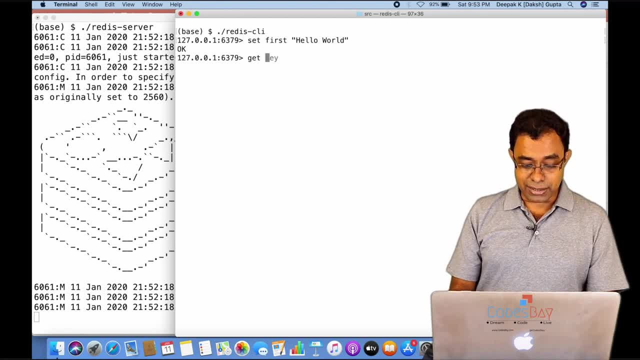 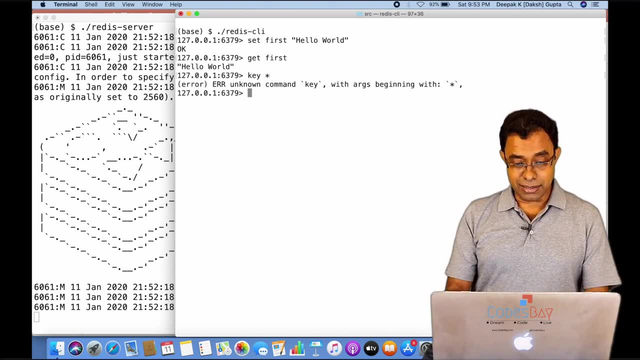 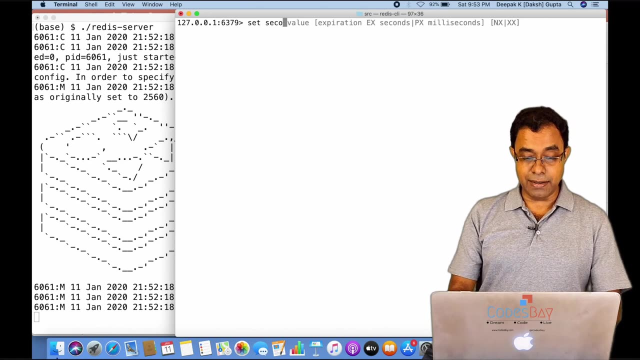 OK means it is being done. If I want to get the key, I can say: get first. If I want to know the keys that are there in my Redis, I'll say keys star, sorry, which is first. I can create one more key called second and I'll say hello, universe. 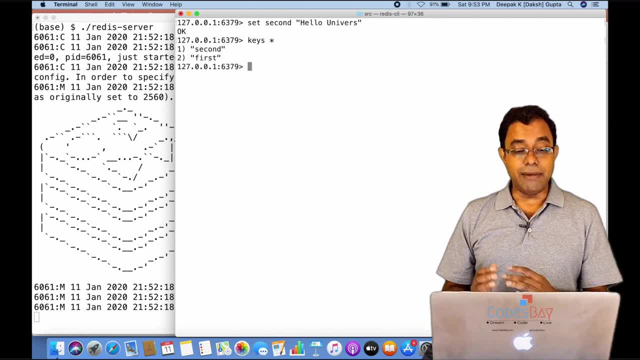 OK, and if I go ahead and get the keys, I will get Both first and second OK. so this is how you can set and get your key value. You can delete a key by saying delete. You say first, Now integer one means it is successful. 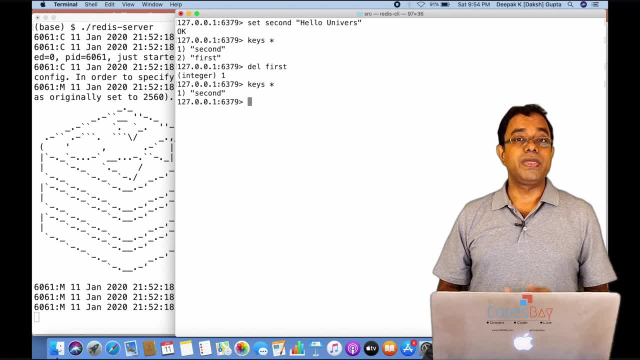 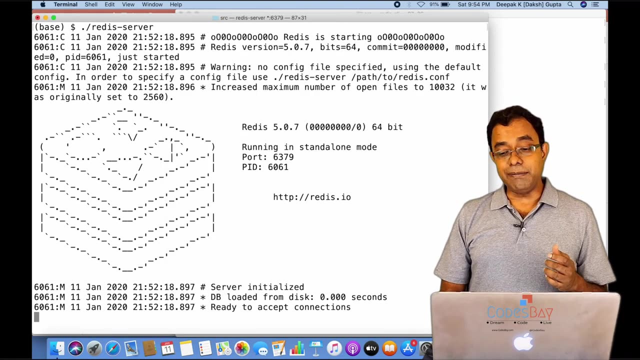 And if you say key star, you will get only second. Now what happens that? let me create one more key first again. Now what will happen is that you know what, When you Close this Redis server and come back again, these keys will not be there.